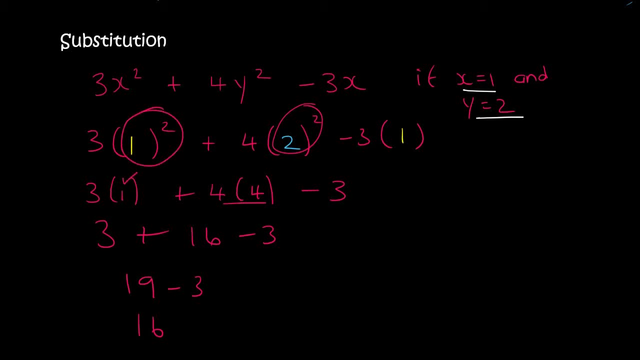 So, for example, you could have done this part on your calculator and then you write the answer there. You could have done this on your calculator and you write the answer there, And then this you can do on the calculator, this you can do on the calculator. As long as you're showing your teacher the smaller steps, then it's fine, You can use your calculator. 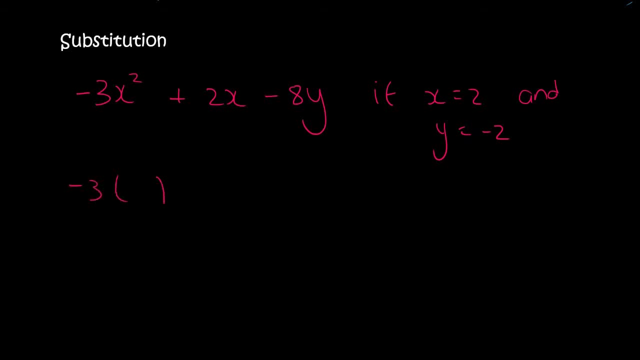 Here's another one. So all you do is you write everything down, You open up brackets wherever you see an x and a y, but you don't change anything else. Like that. If you do it like that, you will get this correct. Now x is 2.. So wherever there was an x, you just go replace it with a 2 and y is minus 2.. Now use your calculator and do smaller parts So you can type that in on the calculator. 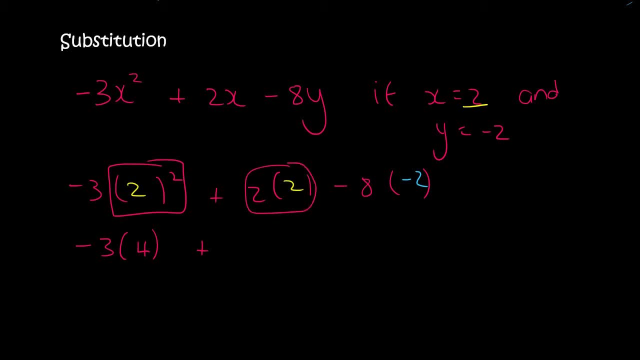 That'll give you 4.. This is just 2 times 2.. So that 2 is a bit high up there, It's down there, so that's 4.. And then you can type in this part on your calculator, going to be my. that's minus over there. so I'm putting a minus over there and 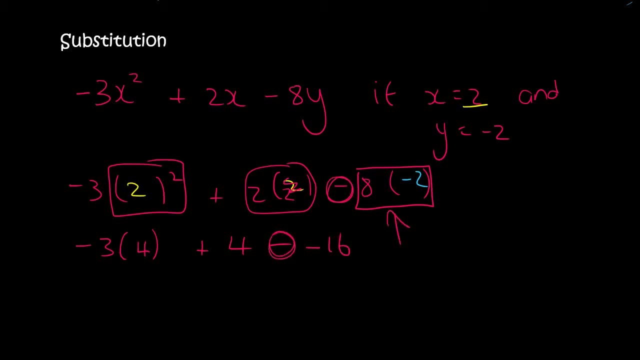 then this part if you do on the calculator, it becomes minus 16. now this you can type in the calculator: that's minus 12, a minus and a minus, that's just a plus if they're next to each other. and now you can do the smaller parts in the 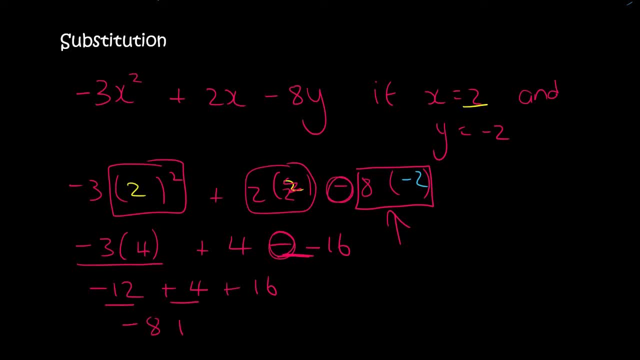 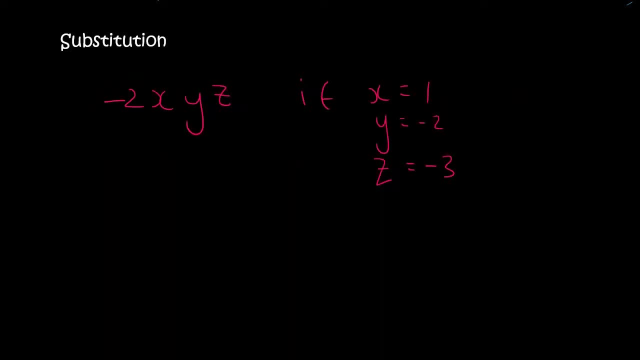 calculator. so you say: minus 12 plus 4, that's minus 8. and then you type in: minus 8 plus 16, and that is 8. so here's another one. so now we've got X, Y and Z. so you open up a bracket for each letter. X is 1, so I just fold that in. 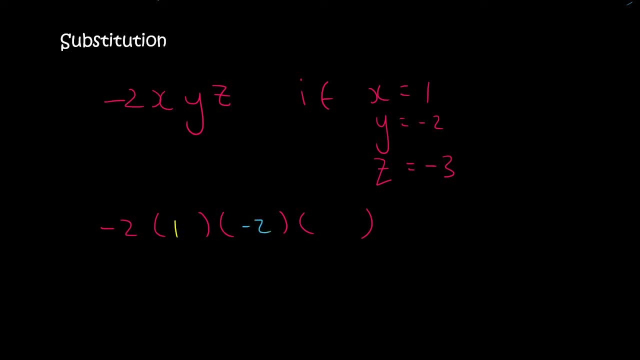 there, y is minus 2 and Z is minus 3, and so this you can simply type in on the calculator: it's just gonna give you negative 12. have a go at this one. so wherever you see Xs and Ys, you can just use a little bracket. so there I see an X. 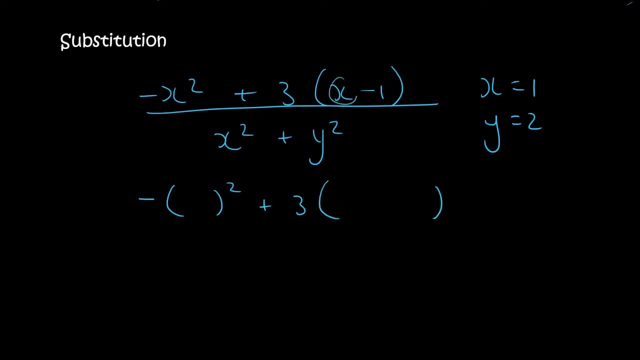 so I'm going to use a bracket here. I've got a little bracket, so I'm going to use a bracket here. I've got a little bracket, so I'm going to use a bracket. so I've got a bracket, so I'm going to use a bracket. 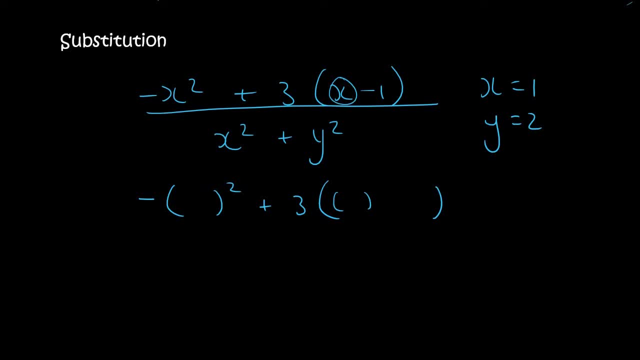 bracket within the bigger bracket, and so I'll do that. and then at the bottom, you just open up a bracket wherever you see an x or y, and there we go. that's the difficult part. notice what I did. I, literally, wherever I saw an x, I just put a bracket. okay, you see that. and then also where 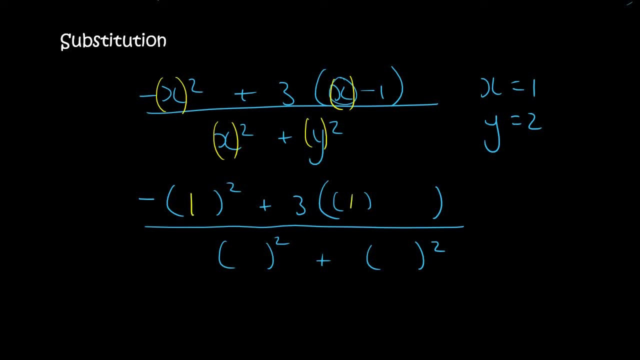 you see a y now x is 1, so you just go fill that in. and then y is 2, so you just fill that in. now you use a calculator, so this part you can just type in on the calculator and that's just going to give you minus 1. oh, I've left out a 1 here, so this part inside the bracket is 1 minus 1, which. 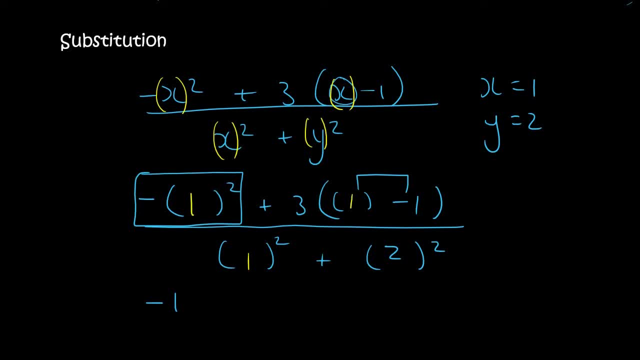 is 0, and so that's just going to be 3 times 0, which is 0. this part here is just 1 times 1, which is 1. this part is 2 to the power of 2, which is 4, and so we end up with minus 1 at the top and 5. 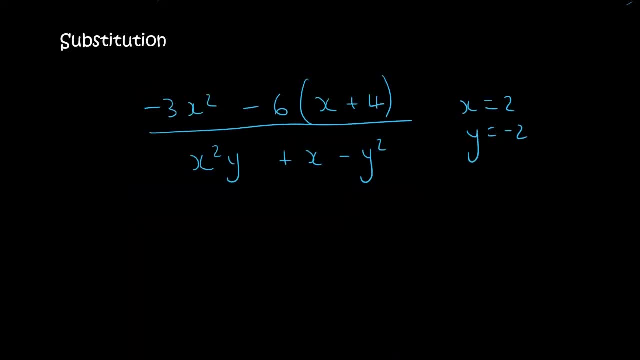 at the bottom and that's the answer. so here's the last one. so x is 2 and y is minus 2. so you just rewrite everything and wherever you see an x or y, you just put a bracket. so notice that this bracket is already there. so, and then for the x I need 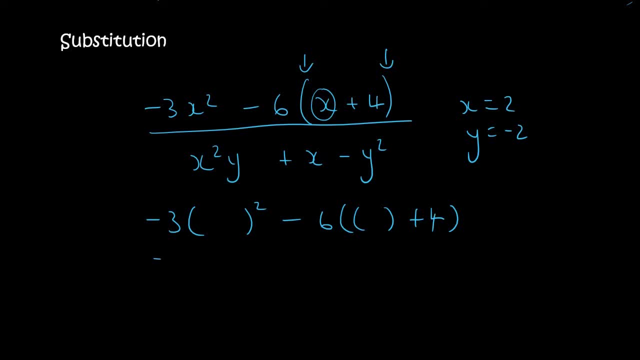 another bracket on the inside. there we go plus 4, then I've got a bracket here. now I don't put the 2 inside the bracket, the bracket is just for the x. and then I've got a bracket for the y, another bracket and another bracket squared. 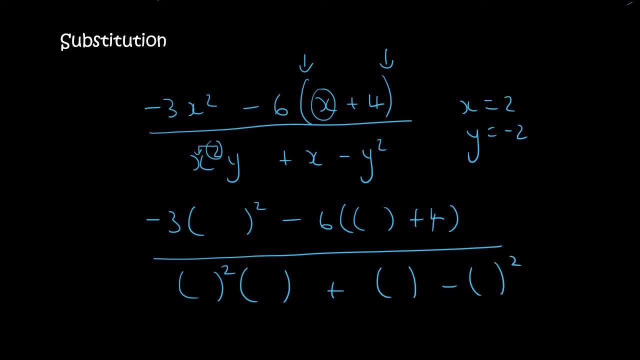 okay, so now. Now I fill in x's or 2 in the place of x. so that was there, there and there, oh and there, and then minus 2 for the y, so that will be this one and this one. 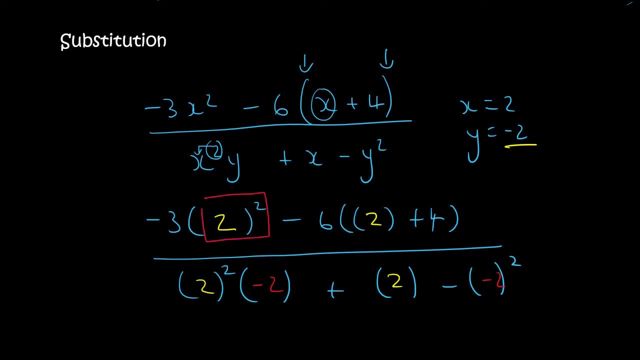 Easy as that. Now here you can do this part on the calculator and that would give you 4, so that's going to be minus 3 times 4, minus 6.. Now inside this bracket it's just 2 plus 4, so that just becomes a 6,. 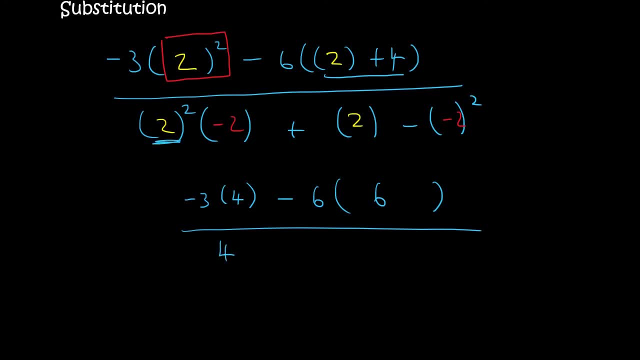 and then at the bottom: well, that just becomes a 4, so you just want to show your teacher the smaller steps. so that part there became a 4, and then this is just plus 2, then this part you can type in the calculator.